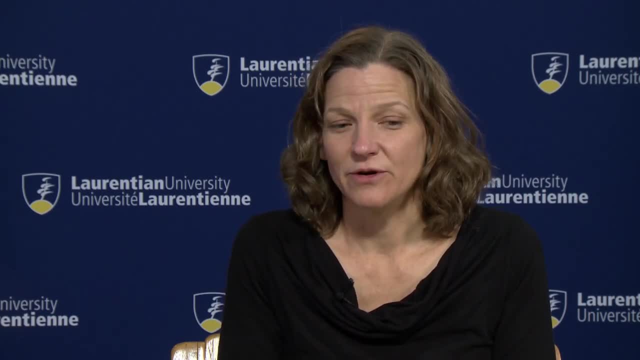 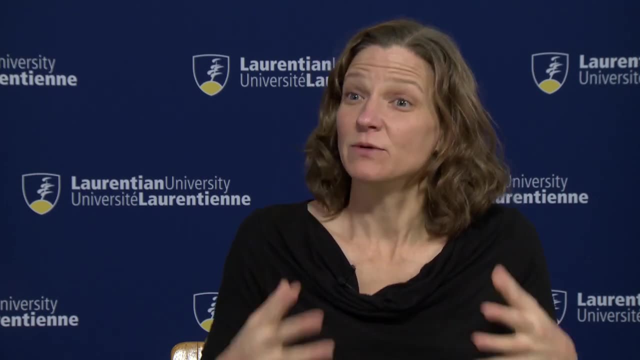 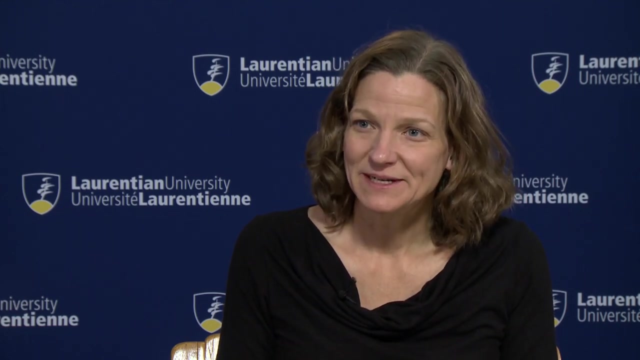 I did a few interviews when we were funding for PermafrostNet and one of the interviewers asked me: so climate change is real then And I was surprised to have that question again. and I think you know, of course, but we're not talking about that anymore Now we're dealing with the consequences. 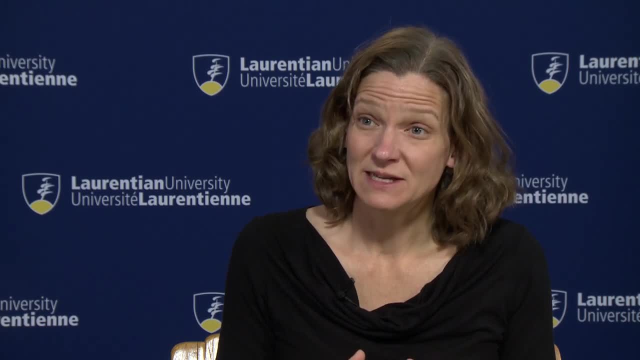 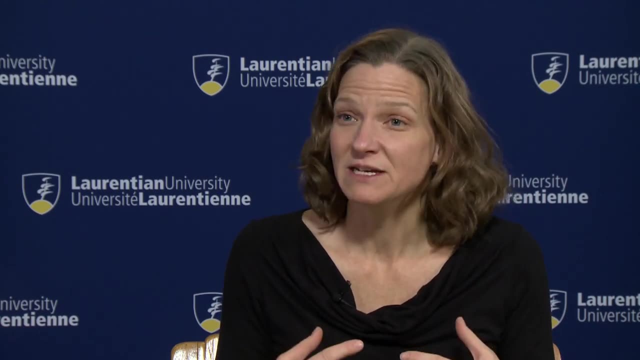 of climatic warming and there are some people for whom that consequence is very real and very threatening to their livelihood and their security and their cultural integrity, and those people are Canadians and it's our responsibility to provide assistance to those people. My name is Pascale. 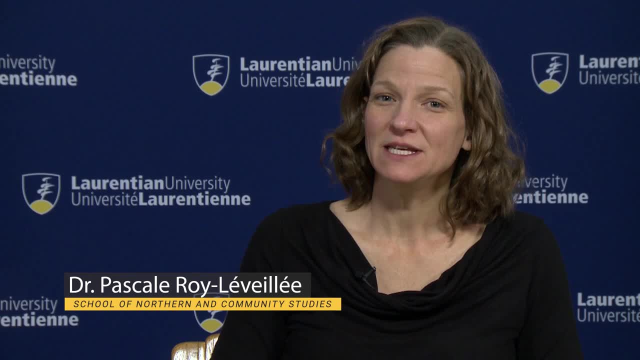 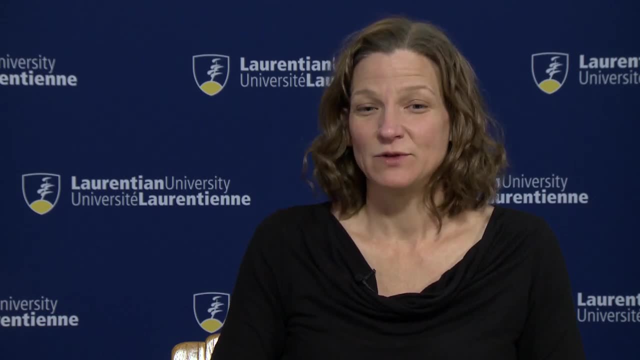 Rouali-Veyer. I'm an associate professor here at Laurentian University in the Department of Geography. I'm a physical geographer and I specialize in permafrost science specifically, so I do my work in the northern part of the country, mostly in the Yukon and in the Hudson's. 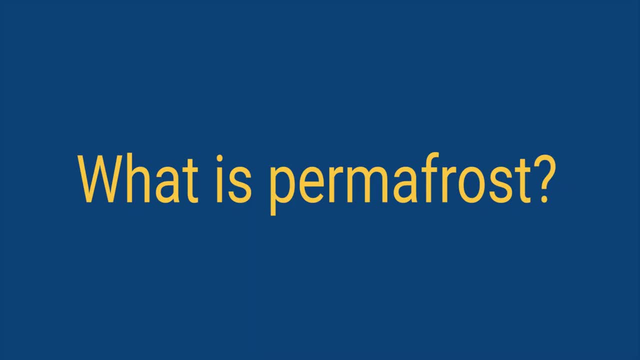 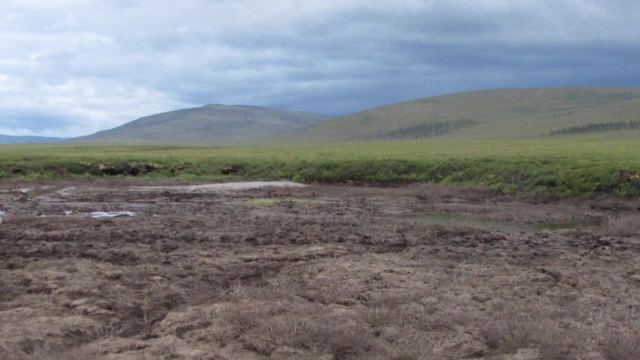 Bay Lowlands also. Permafrost is ground that has been at or below zero Celsius degrees for two or more years, and that sounds a little bit technical, but it's because permafrost sometimes is frozen, meaning that you know it's. 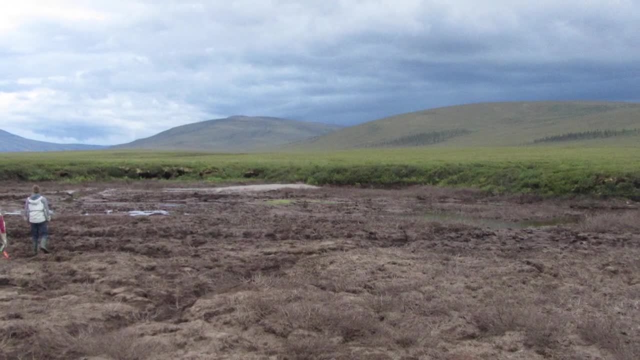 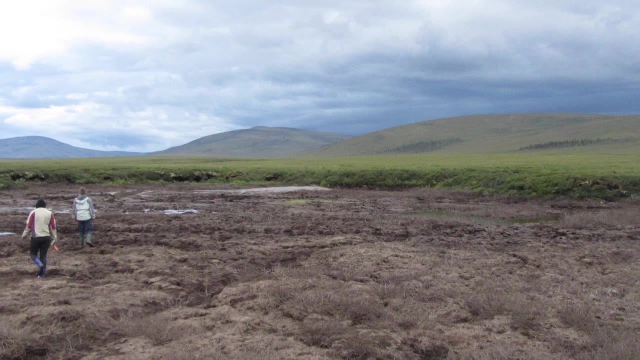 wet ground that has water in it and has turned to ice. That's mostly the kind of permafrost that we're interested in. actually I'll talk more about it in a minute. but technically permafrost could just be solid bedrock that is below zero Celsius degrees and has no water in it and that. 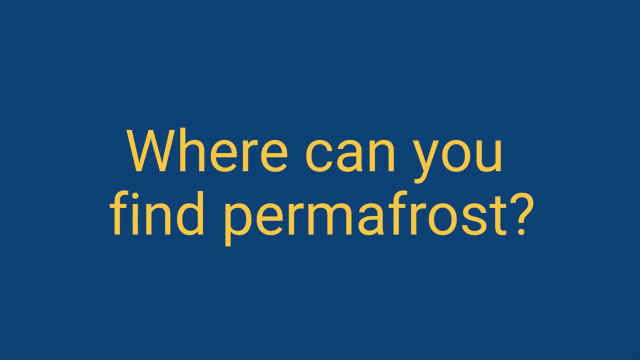 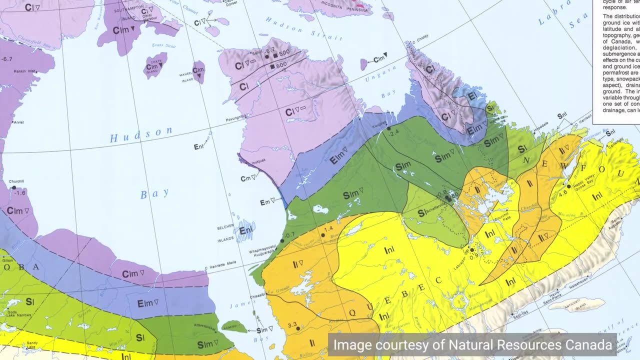 counts as permafrost. also, Half of Canada's landmass is included within what we call the permafrost zones. so it's not quite correct to say that half of Canada is under landmass, but it's pretty much the same by permafrost. But in half of Canada we might encounter permafrost below the. 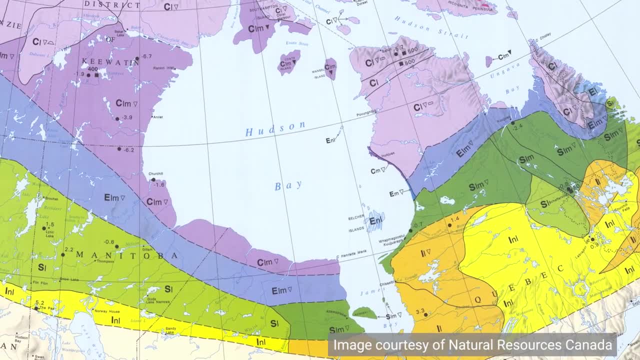 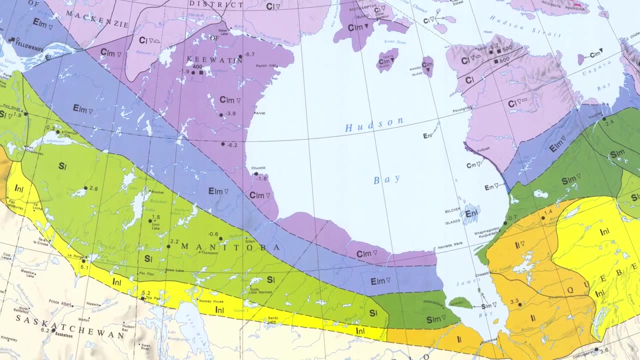 ground. So when we move further north we have what we call continuous permafrost, meaning that we expect to have permafrost pretty much everywhere. And then as we go further and further south in the permafrost zones, we start having this continuous permafrost that eventually becomes sporadic. 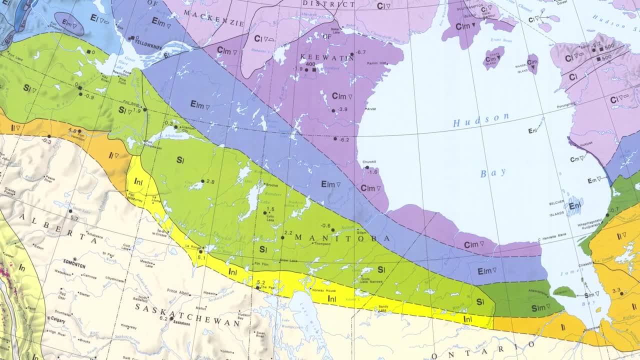 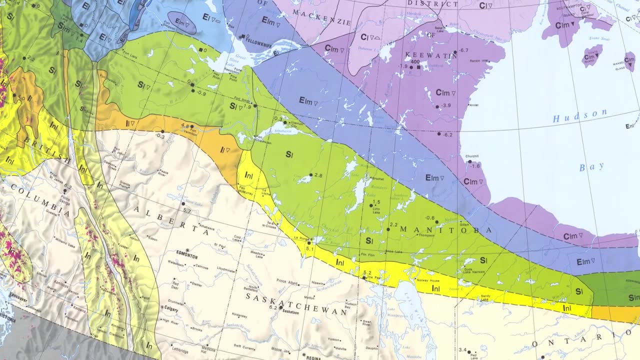 where we have just isolated patches at the very southern limit of permafrost. So half of the country is affected by permafrost, could have permafrost beneath it, a lot of it further in the north And then, as we go further and further south or in areas that are progressively 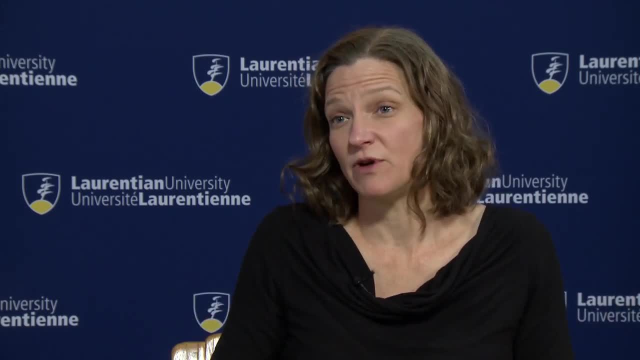 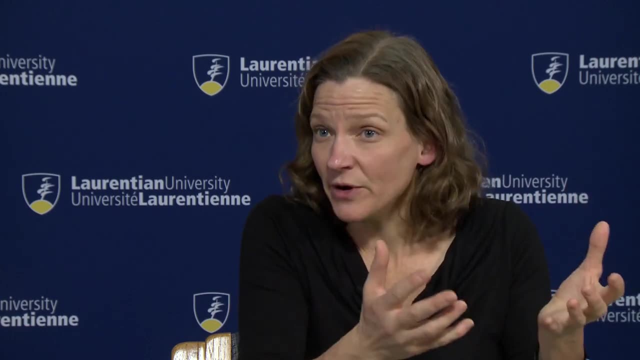 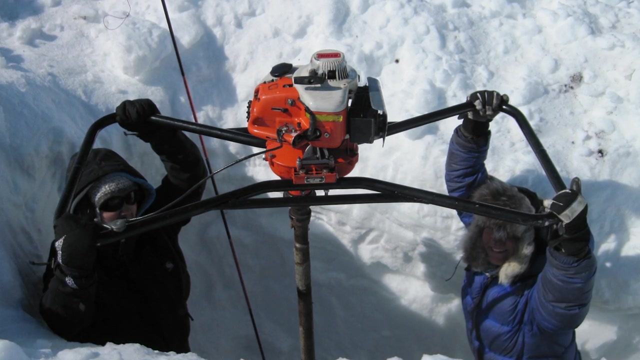 warmer. we have less and less of those occurrences of permafrost or frozen ground beneath the ground surface. Further north in the Arctic part of our country, where we have cold mean annual air temperature, we'll have cold ground temperatures also. So in those areas the progressive warming 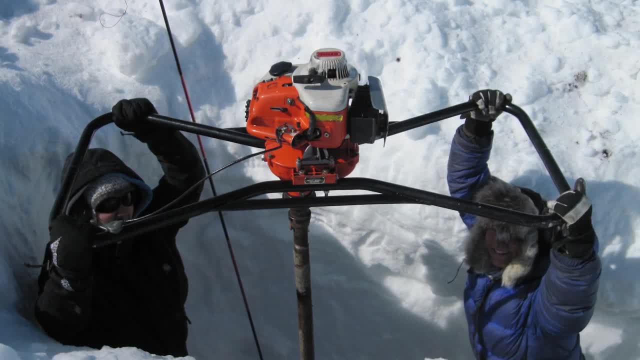 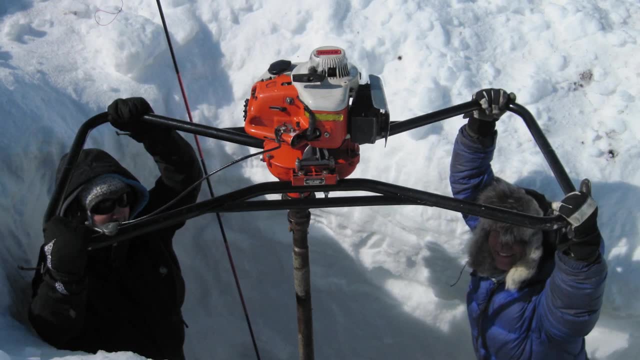 of climate and changes in precipitation patterns is having as a result increasing the average temperature of permafrost progressively towards zero. But as we go further, in those areas that have just patches of permafrost, those patches often have an average temperature that's. 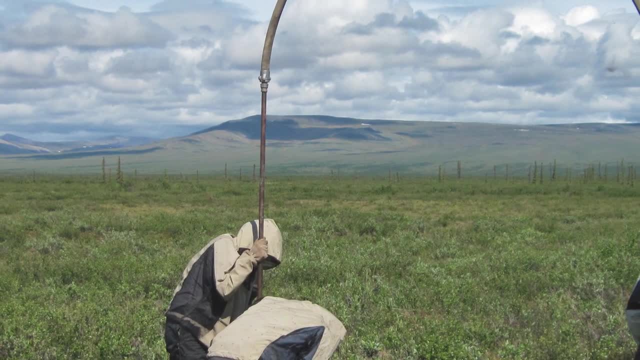 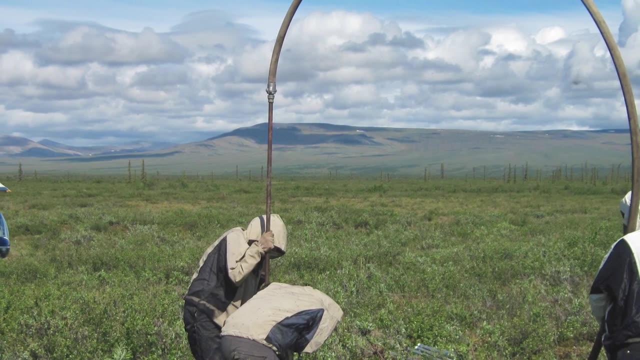 pretty much at zero Celsius degrees already, because it's just at the limit of where it can be sustained. And then, as we're increasing its temperature, as we're putting more heat into the ground, then those patches of permafrost are thawing progressively. In areas where the permafrost 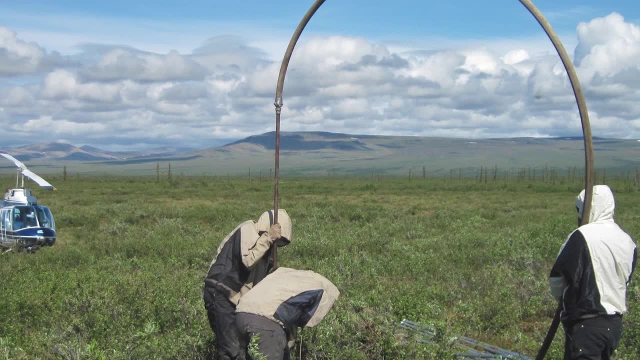 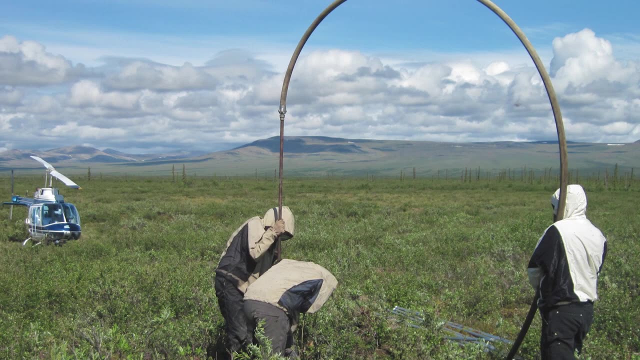 is so in between, I guess, those isolated patches and the very cold area where the mean annual warming, then we have areas where permafrost can still be sustained even under warming conditions for now, but often the layer of ground above permafrost there's always a. layer there that freezes and thaws every year. That's where plants put their roots into the ground. So that layer of ground, which we call the active layer that freezes and thaws every year starts to be deeper and deeper And we're starting to lose some of the permafrost. via the top of it, as there's a deeper and deeper layer that thaws into the summer. So thawing of permafrost happens in different ways. I guess Near the south those patches can disappear. In areas where the permafrost is thicker, it progressively can thaw from. 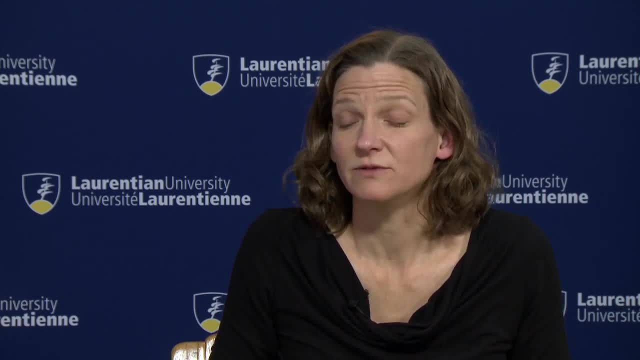 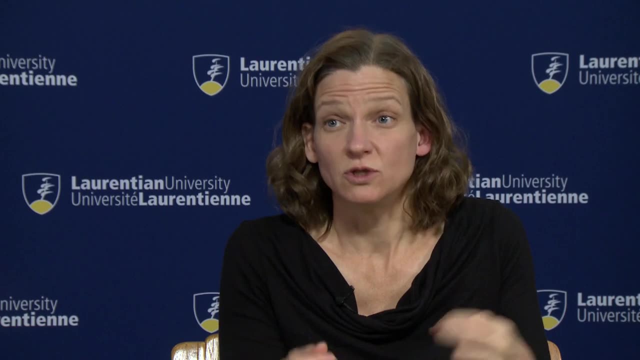 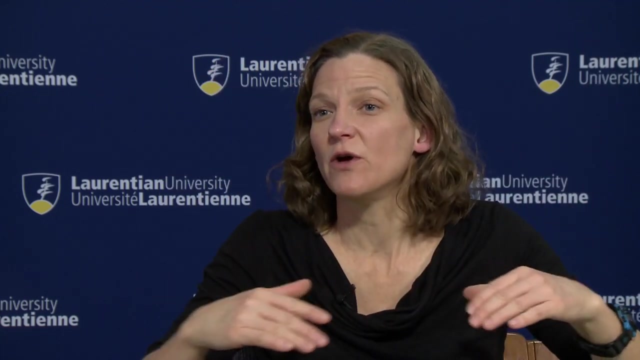 the top, which sometimes can happen very fast because it affects the ground surface when it starts to thaw. So there's two key drivers of permafrost research, two main problems that we have when permafrost thaws. One of them is that the areas- half the country, the areas that are in the permafrost zones- that are affected by permafrost contain a lot of carbon in the ground. By carbon in the ground I mean dead plants and dead animals, also potentially dead living tissue that has been into the ground and normally elsewhere that would decompose, But in permafrost areas that dead organic material has been. 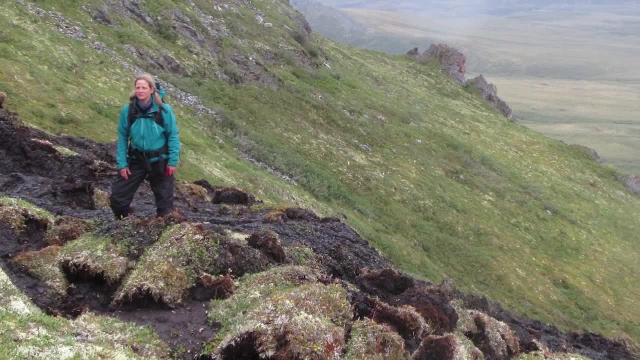 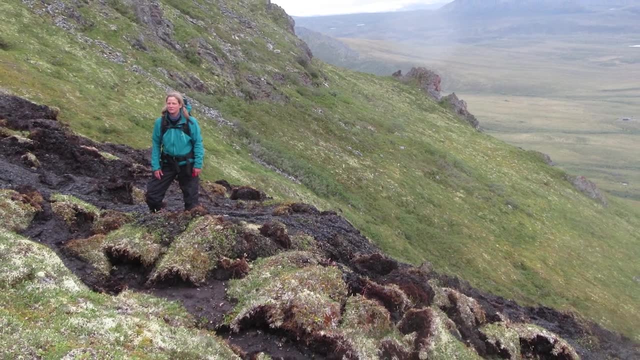 – it's like it's in the freezer, So it's been preserved from rotting, from decomposition by the cold temperatures of the ground It's frozen in, And now, as the permafrost starts to thaw progressively, all of that living material can now thaw. 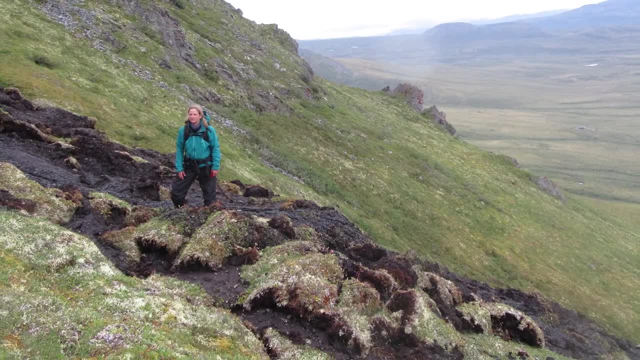 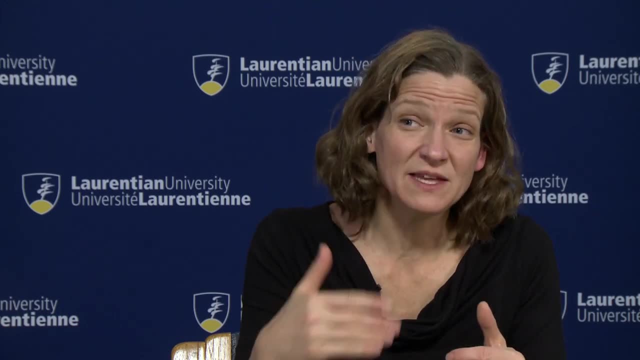 All of that living material can now start to rot and decompose And then as it rots it emits greenhouse gases, So carbon dioxide and methane also, which is a very potent greenhouse gas. So the potential feedbacks there to climatic warming. you know, you warm up the climate. 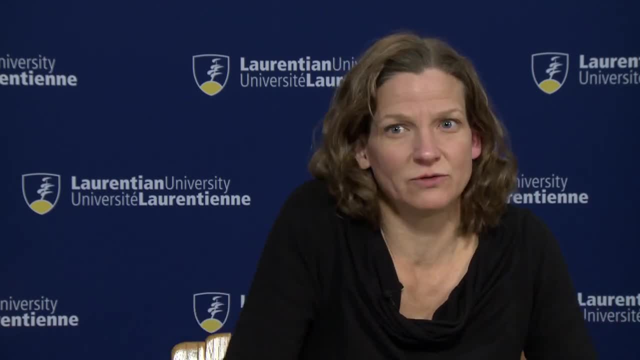 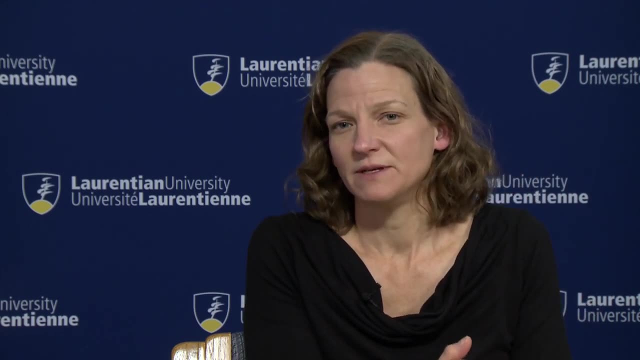 a little bit, permafrost starts to thaw, that organic material starts to rot, a bunch of methane and carbon dioxide comes out of the ground. People are very concerned about this potential feedback to climate warming. So that's the first driver, or one of the key. 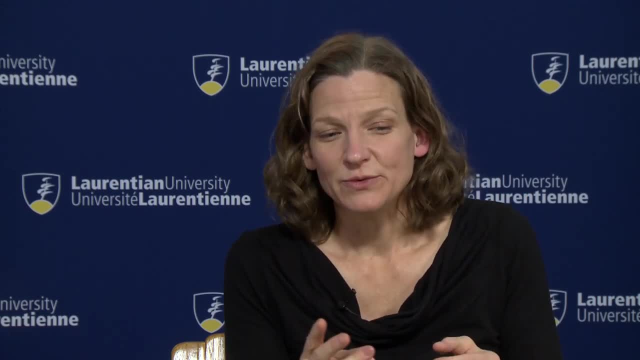 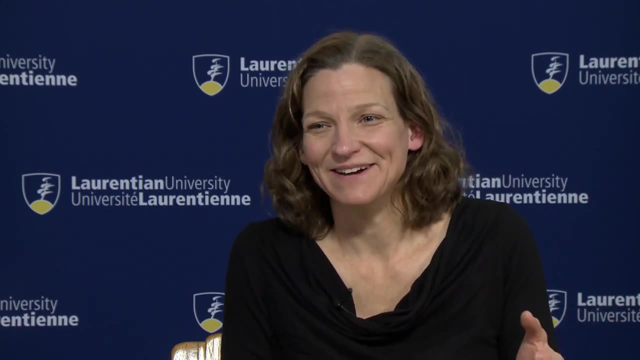 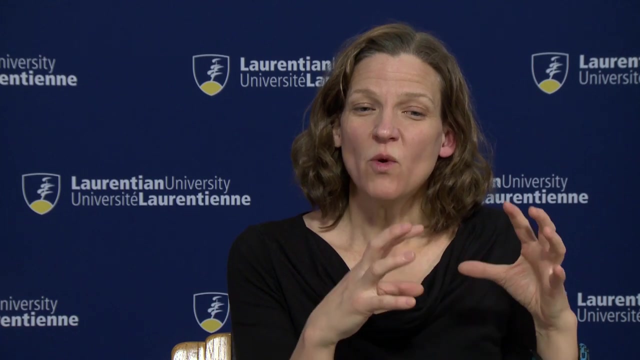 driver of permafrost And then the other one. the other, I guess very important one is that in permafrost we have a lot of ice also, Not just living dead plant material, but we also have a lot of ice in permafrost. In fact, we have a little bit more water held in permafrost. There's sometimes a lot more water held in permafrost than what the pore space of the ground can hold once the ground has thawed. Which means that if permafrost thaws you get regular ground mud settling sort of at the bottom. So it's a lot more water held in permafrost. And then there's all this extra water that now has to go somewhere. So you get very muddy conditions on the ground, You get a loss of volume, a loss of physical properties, but you'll also get things like big ponds and lakes forming at the surface if it's a flat. 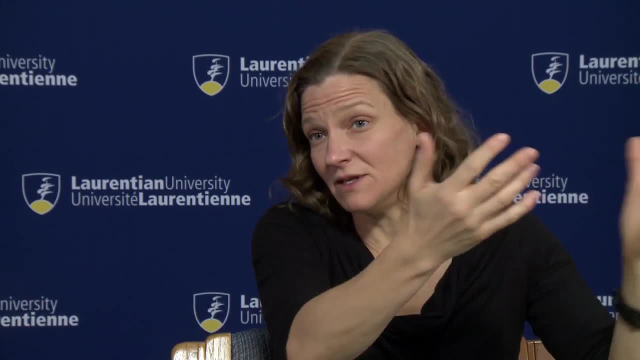 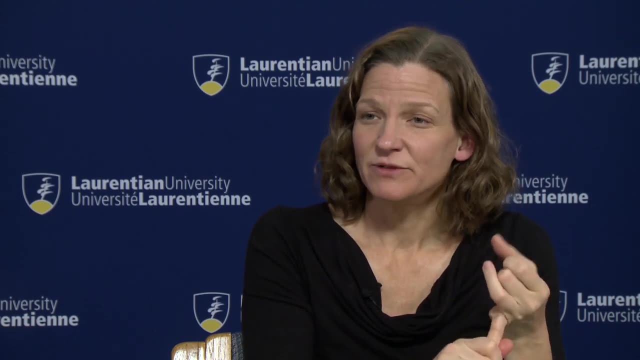 area that's thawing, Or if it's on slopes, you get landslides and different kinds of mass movement resulting from the ice on the ground thawing. So the carbon in the ground and the feedback to climate is one of the main problems associated with permafrost thawing. 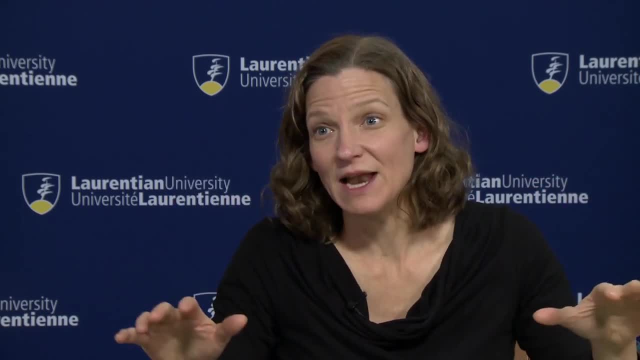 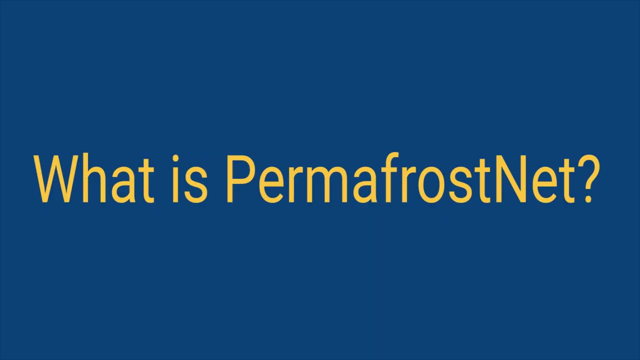 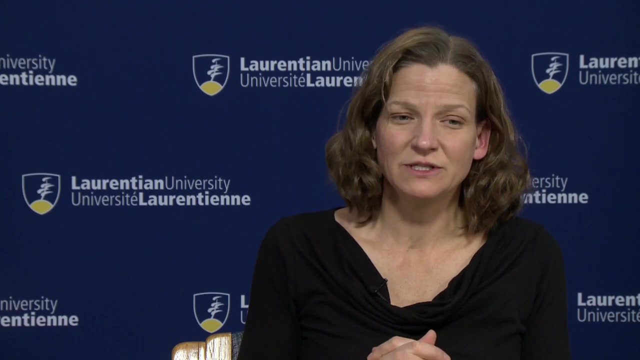 Speaker 2 And the other one is all the ice in the ground and the ground surface collapsing as those chunks of ice are melting when the permafrost thaws. PermafrostNet is a Canadian network of permafrost researchers that include a lot of permafrost scientists and permafrost engineers also, and it's focused specifically 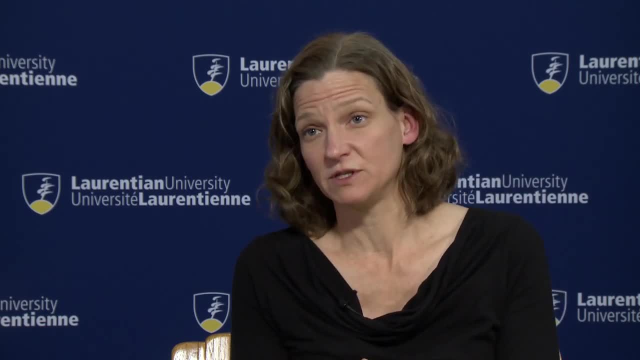 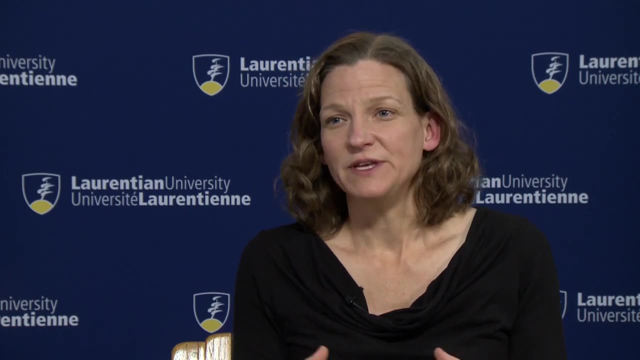 so the purpose is to help Canadians and Canada prepare for permafrost thaw. The focus of PermafrostNet is specifically permafrost as a structure, if you will. so the impacts of permafrost degradation on the land surface resulting from the degradation of 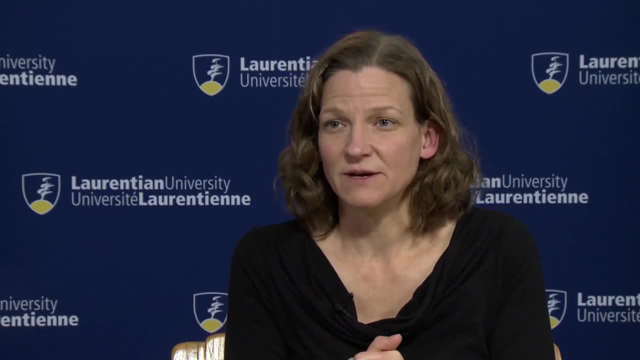 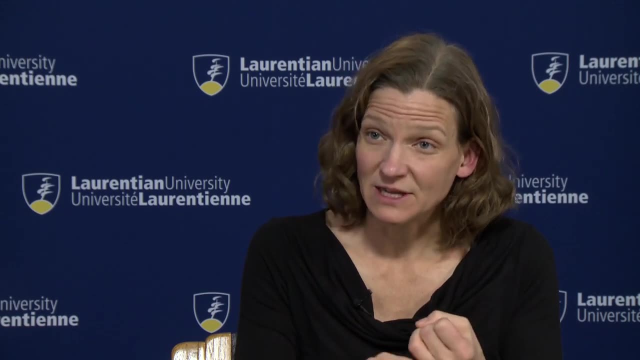 ground ice in particular is what PermafrostNet is focusing on. So there's different aspects in PermafrostNet. it's interested in first of all, improving the mapping of permafrost and the characterization of permafrost. Canada is a big country and there's patches of permafrost that 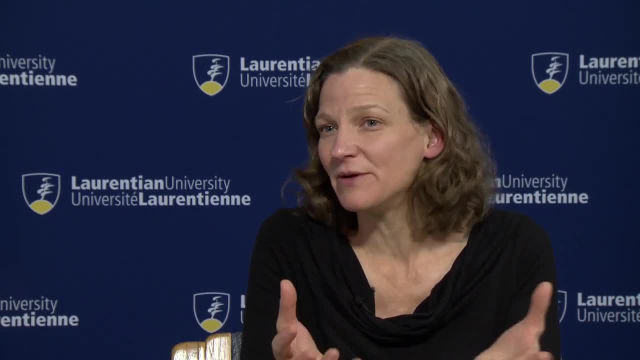 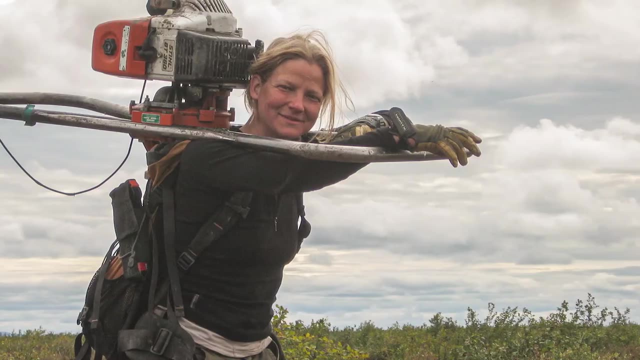 have been very where there's been very little studies, areas where we don't know the conditions very well- how thick is the permafrost, how cold is it and how much ice is in it. So there's a whole component where we're trying to fill those. 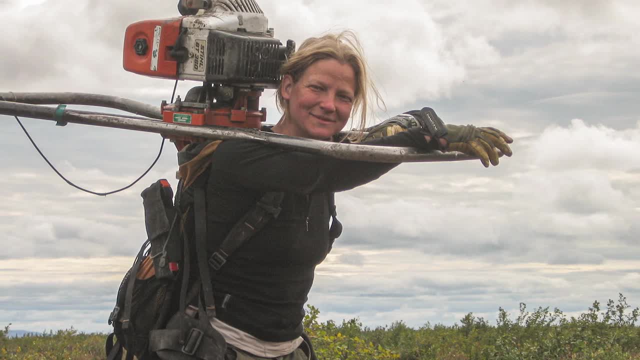 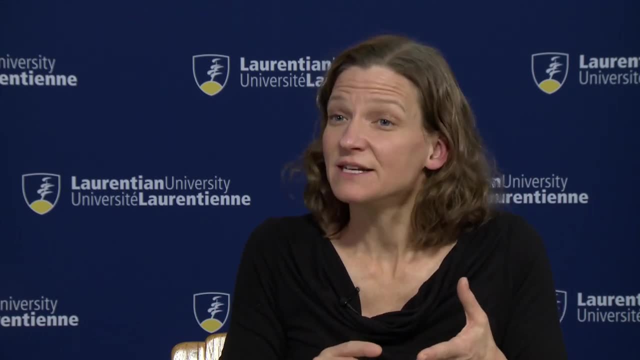 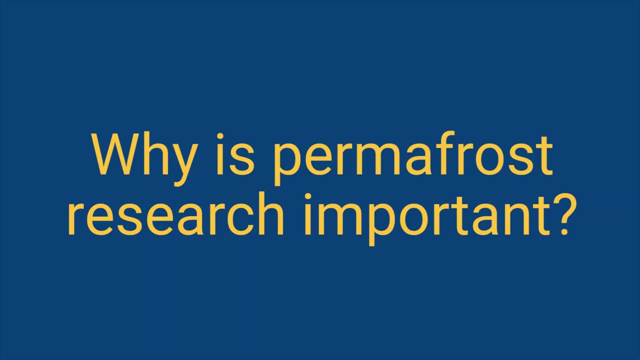 data gaps and then after that there's a monitoring component to try and develop ways to better monitor how permafrost is changing over time, and then identifying the hazards related with permafrost degradation and adapting to permafrost degradation. I was really happy when 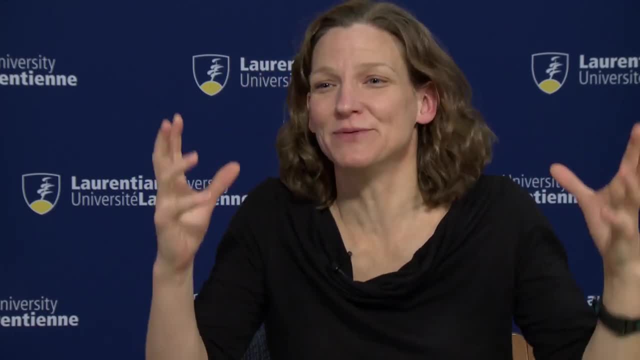 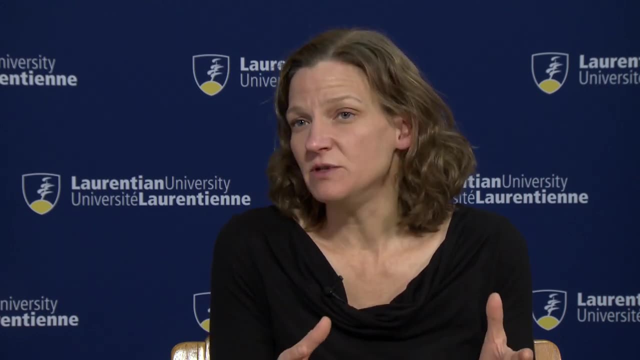 PermafrostNet got funded not just for personal career reasons, right like I really thought that it was the right decision and that it was the right thing. PermafrostNet, so the permafrost science community, is not that big. it's a specialty topic, if you want, in a sense. 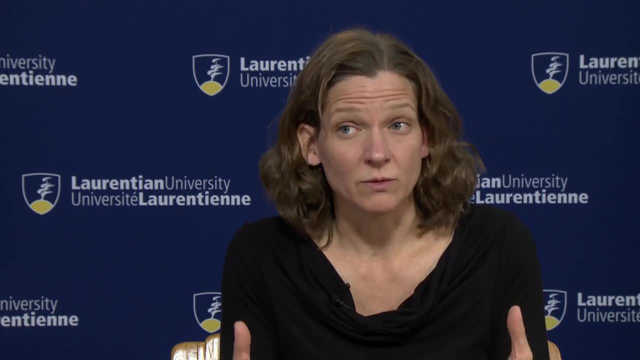 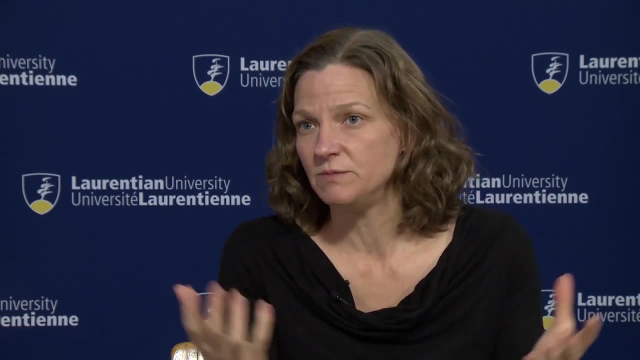 and there's people studying permafrost and permafrost degradation all around the world, even in countries where there's no permafrost. So one of the biggest research centers, for example, is in Germany and you know, there's people all over the place studying permafrost, People who come 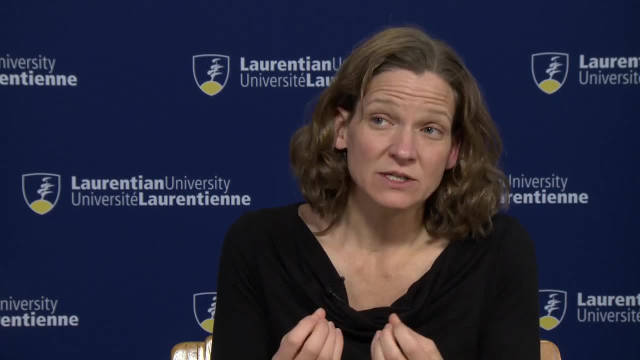 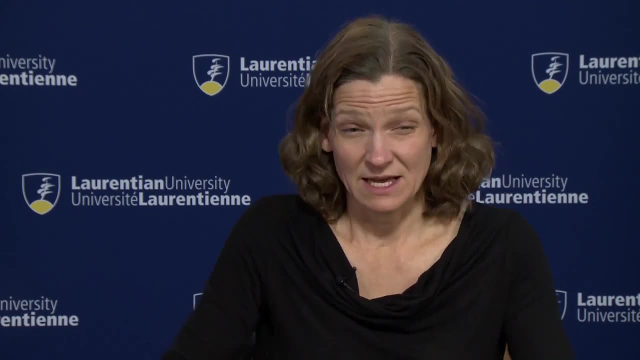 from countries where there's no permafrost. there's a lot of people who come from countries where there's no permafrost have a particular interest in global change and the potential positive feedbacks to global warming. right, As I said at the beginning, when permafrost degrade, it can have. 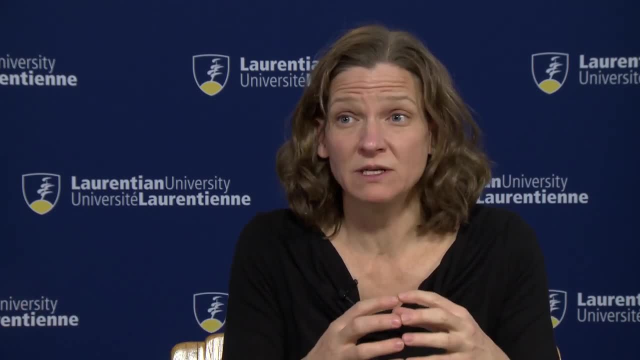 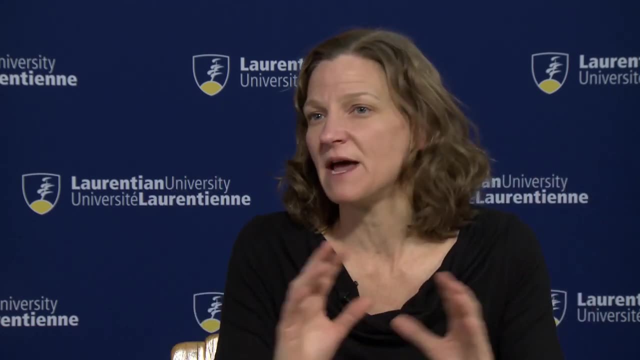 feedbacks to accelerate climatic warming. This is really poorly integrated in our global climate models at the moment. It's kind of an emergency. we're not doing this well and it could have big, big impacts, and people around the planet are worried about this, So they have their eyes. 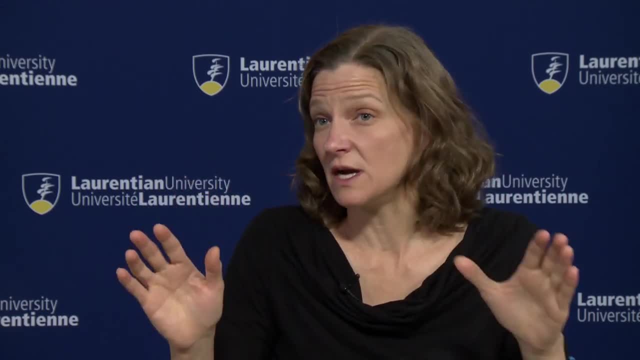 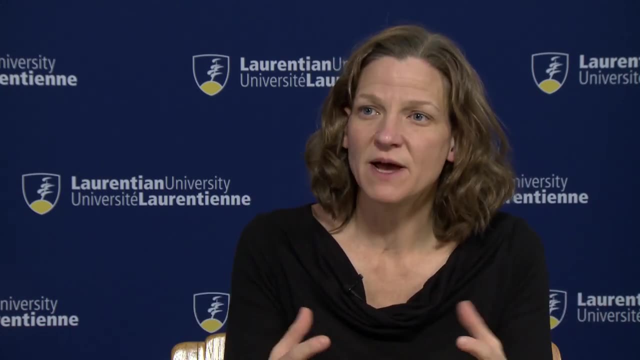 on places like Canada where permafrost is thawing, and they want to know what's going to happen to all that organic matter. So internationally, and of course in Canada, it concerns us also. there's a concern for the climatic feedback and there's quite a bit of 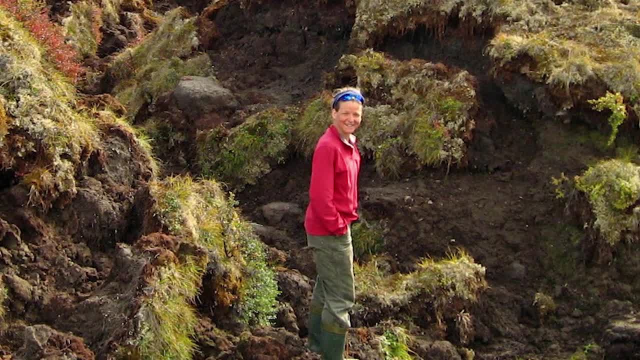 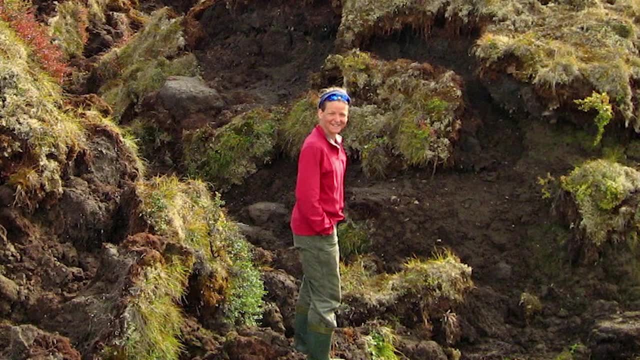 attention being put in that at the moment In Canada we also have communities and people who are living on permafrost right and who are working on permafrost. That's the areas, that's their land, that's where they have their communities, and these people are affected. 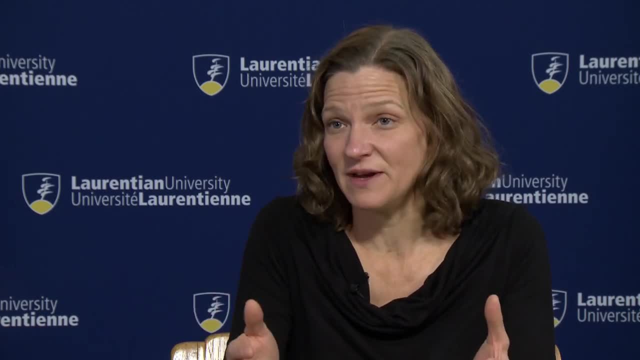 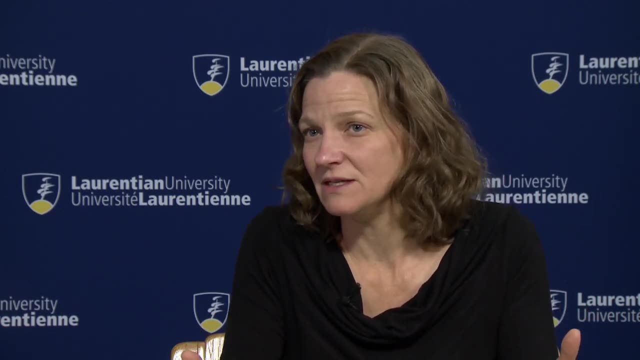 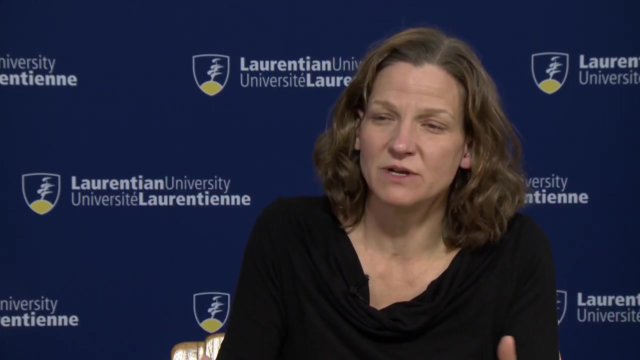 in a different way, if you will, although climatic feedbacks will affect them, But in the immediate future, ongoing at the moment is just the fact that the ground is thawing beneath them and their houses, you know, not falling in the hole, but cracking and being damaged by the degradation of permafrost and 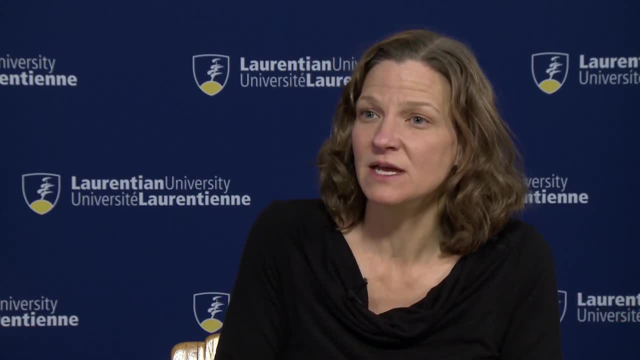 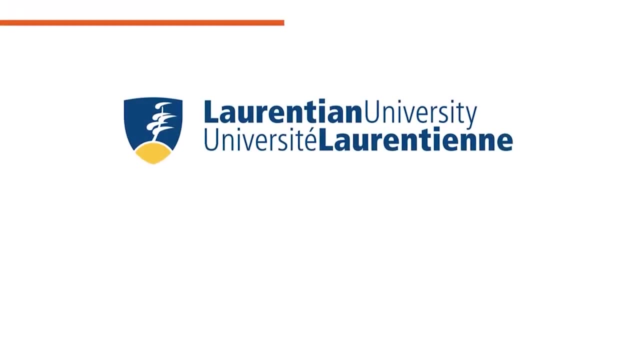 the road to work is threatened by a slump that's moving towards the highway and you know there's like very concrete and urgent consequences of permafrost degradation and climate warming for those people.